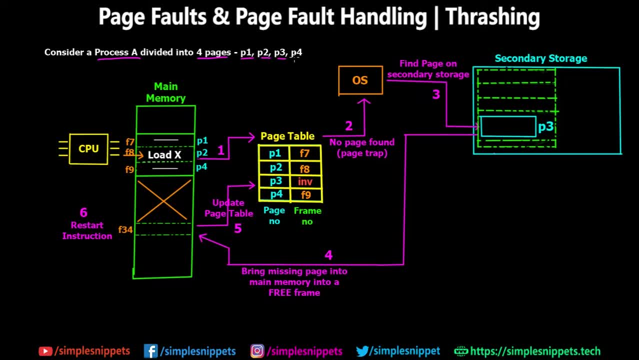 is process A and it is divided into four pages: P1, P2,, P3 and P4.. Okay, So since process A is very big and our page size is small compared to process A, we have to divide this by the process in four pages. and we already know: in paging the virtual memory is divided into 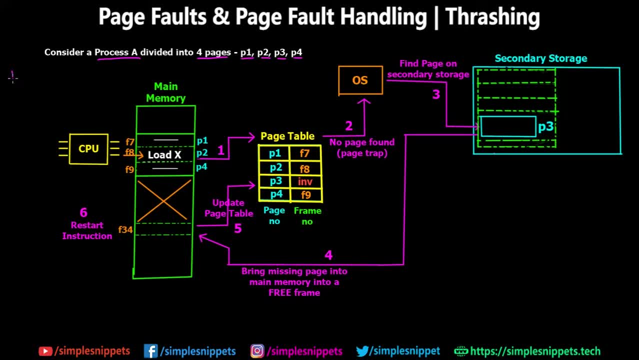 pages and the main memory is divided into frames, and pages is equal to frames, Right, Okay? So what happens in a page fault? So, basically, a page fault happens when a desired page which is about to be executed or is required is not there in the main memory, but it is. 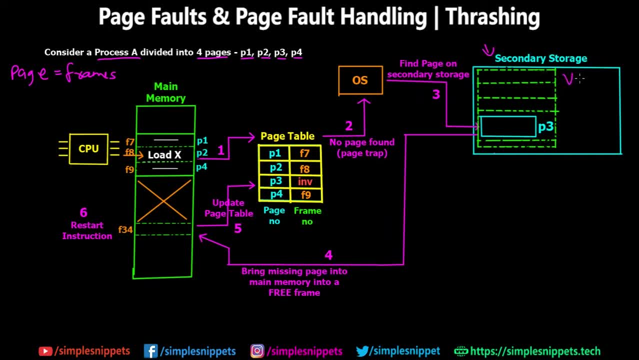 there in the secondary storage or the virtual memory. Okay, So that's what paging helps us achieve, Right? So we create some space in the secondary storage which can be used to store some pages of certain processes if the main memory gets full. Right, So that's how we expand the. 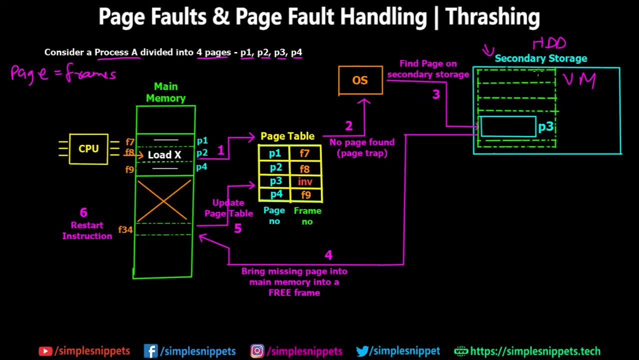 main memory by using some virtual memory. Basically, it is using the secondary storage itself, Right? So now let's consider this situation. Our CPU is over here and it is executing P2, that is, page number two of this process A, and there's an instruction inside this page. 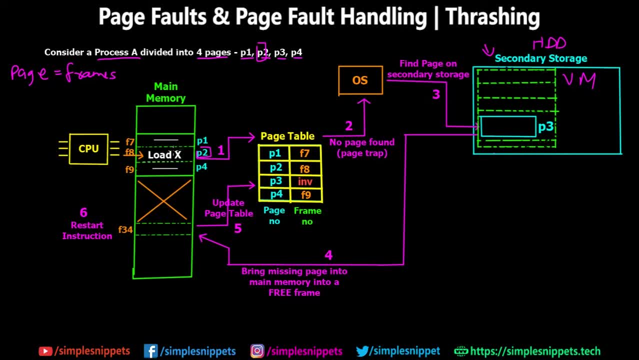 P2, which is load X. Now let's assume that this load X basically requires P3.. Okay, Process 3.. So the CPU will initiate a request of P3, page 3.. So our CPU doesn't know that P3 is not there in the 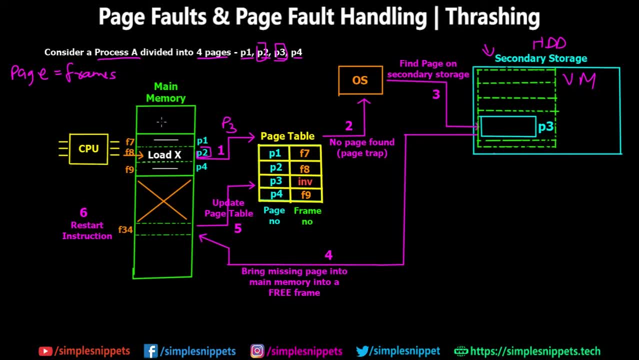 main memory Right. So somebody has to tell the CPU that it is not there in the main memory Right. So this is done by the MMU, that is memory management unit. So MMU will take P3 and look into the page table of process A. So every process has its own page table. 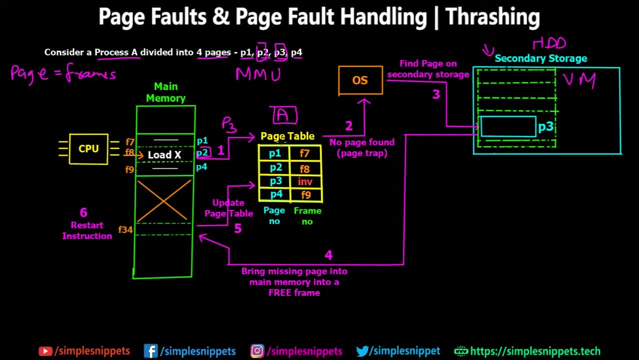 We already know this. So this is for process A. So inside this page table the memory management unit will see: okay, it's P3. So it will directly go to the entry where P3 is there. So this P1,, P2,, P3, and P4 will already be there and corresponding to P3,. 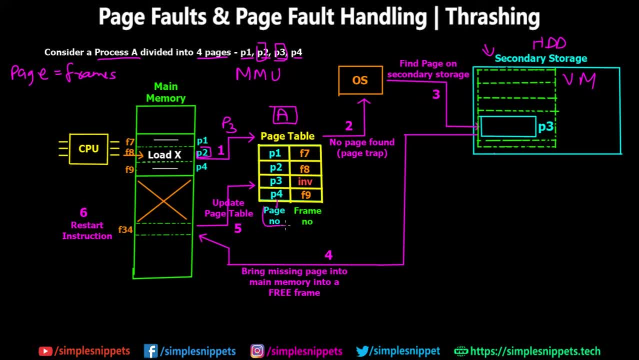 it will see what is the frame number. So this first column is page number and second column is frame number. Now over here you can see for P3, it sees that there is an invalid entry, that is ibit. It is also known as invalid bit, which essentially means that P3- that is 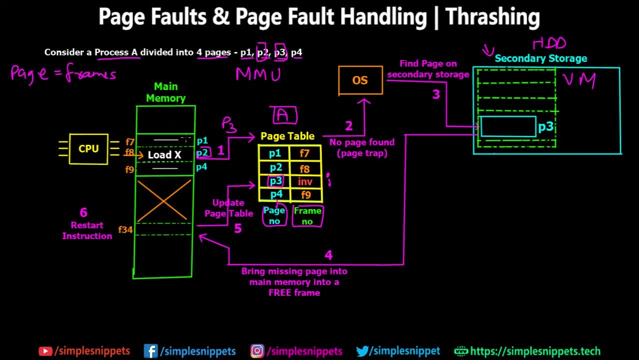 page 3 of process A is not there in the main memory. So you can see we have P1 over here. So this is P1.. This is P2 just below it, and then we directly have P4.. We don't have P3.. 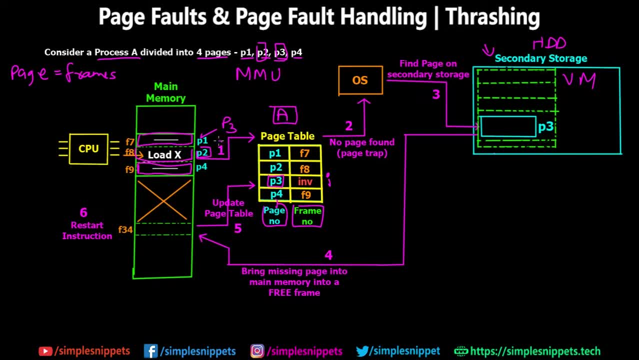 So now what happens is: so this was step number 1 that is looking up in the page table. So step number 2 is a page trap signal is generated. So basically what happened here happened. So we just saw what is a page fault, that is, P3 is not there in the main. 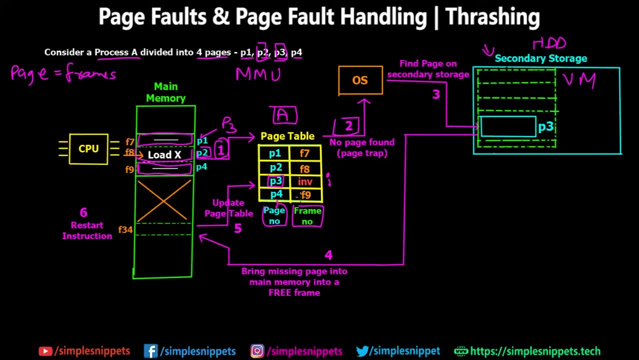 memory, which is a page fault, and we just found that out by using the page table. So a page fault has happened. So I hope you know what is a page fault. Now how do we handle this? So this entire diagram is basically the page fault handling diagram. So we are at step. 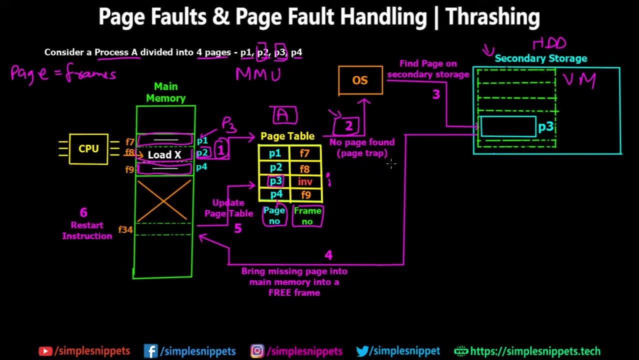 number 2 now. So this is where a page trap signal is generated. So a trap is basically a high priority signal in operating systems which the OS cannot preempt. So whenever a signal which is a trap signal is generated, the operating system has to. 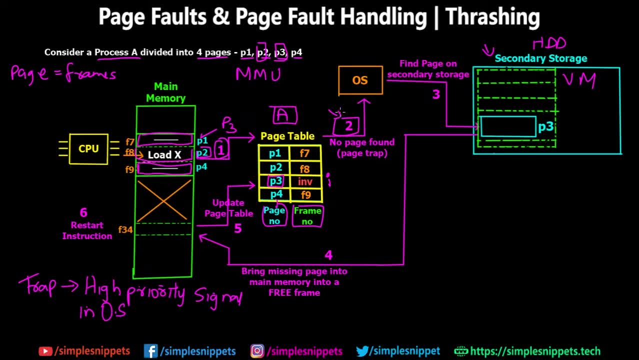 compulsory look and resolve that signal or resolve that query. So just remember that a trap is a very high priority signal which the OS cannot ignore. So a trap is generated and sent to the OS with all these informations that P3 is not there in the page table of. 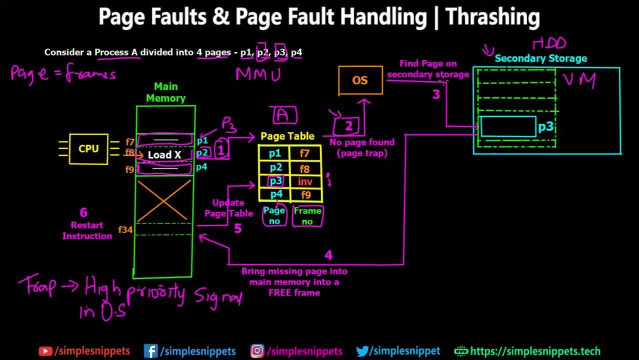 this process A So now the OS has to find the page on the secondary storage which is used as virtual memory. So, using this paging scheme, we have used some portion of the secondary storage as virtual memory right and we have divided it into pages. so this is page for one slot. 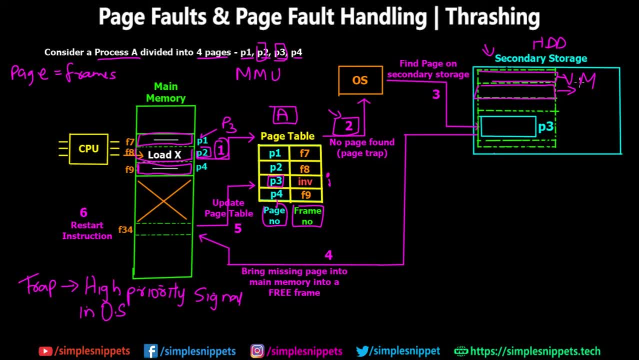 so this is the second slot, and so on and so forth. so somewhere on this virtual memory we have p3. so operating system goes on to this secondary storage and finds out p3 is over here. and then step number four is to bring back the missing page into main memory. 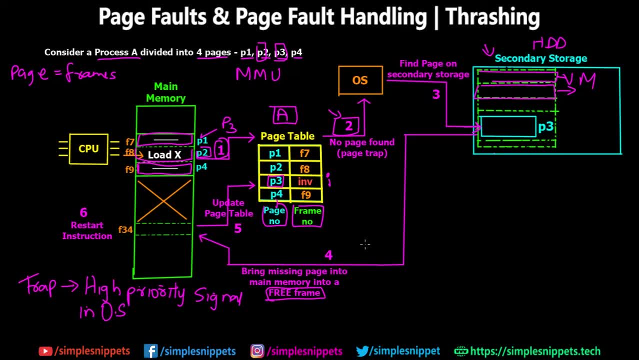 into a free frame. okay, so now the operating system has to check whether there is some empty frame in the main memory and, depending upon where the frame is free, this p3 is being loaded over here. okay, so now p3 is gonna be loaded into f34, because f34 is free, you can. 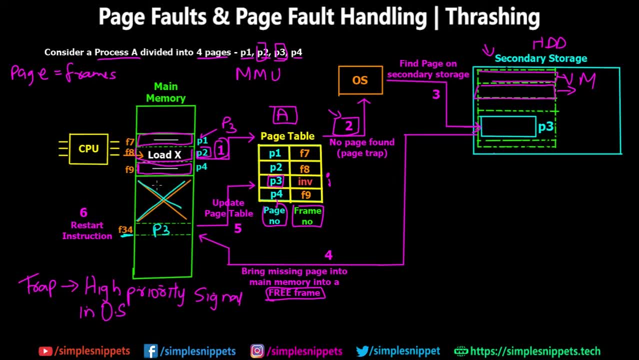 see this cross mark, which means that this much amount of memory is not free over here and directly, the frame number 34 is free. so since this frame size and this page size is the same, it will be directly loaded into this frame number 34. okay, now you realize that. 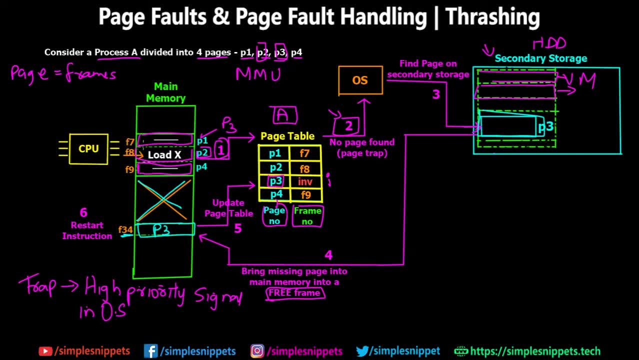 you can see that p1, p2, right below each other in the memory, at frame number F7 and F8.. However, P3, which comes after P2, is being loaded at F34, which is not contiguous right. So this is how paging technique. 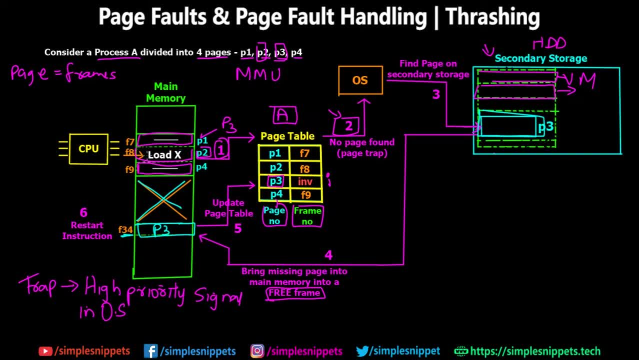 helps us achieve non-contiguous memory allocations. So you can see that it is not needed that P1, P2, P3, P4 be in line. So you can see after P2 we directly have P4, but P3 is loaded. 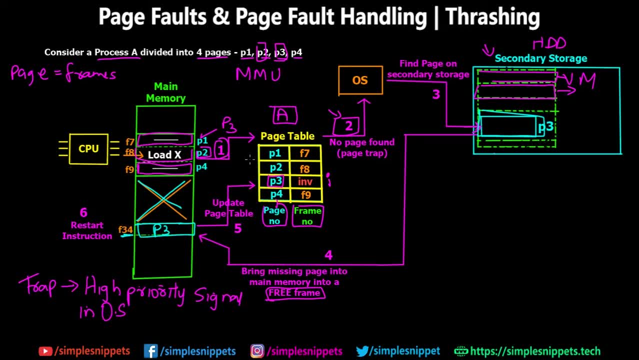 somewhere over here. and the reason why we can do this is because by the use of page table. So we don't need to have P1, P2, P3, P4 back-to-back or contiguous, because in the page table we are directly storing where exactly P1 is, where exactly P2 is, where exactly. 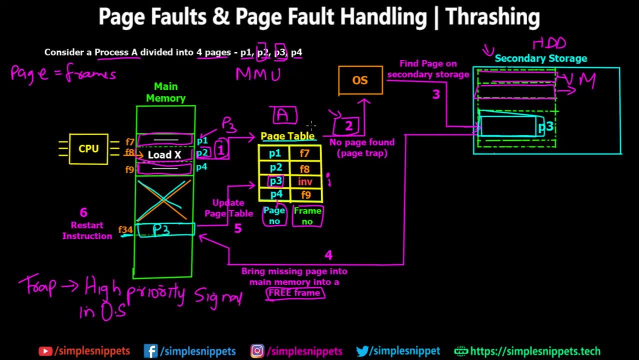 P3 is right, So we are directly having the address and this is why page table acts as an index. So for step number 4, what we did is we loaded P3 in the main memory. and now for step number 5, we have to update the page table. So, by updating page table, what we 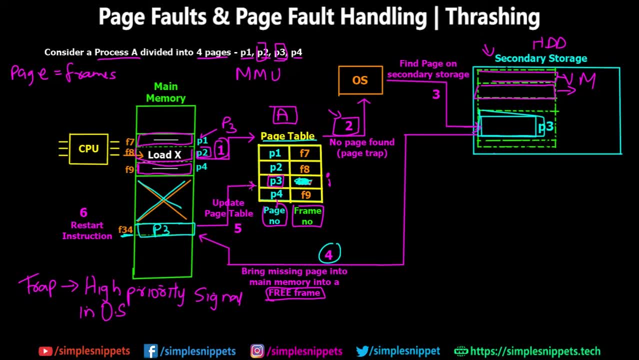 are going to do is we are going to be adding an entry over here, and that entry is going to be the frame number in which P3 is loaded is loaded. so this is now going to be f34. so step number five is complete. and last step of this: 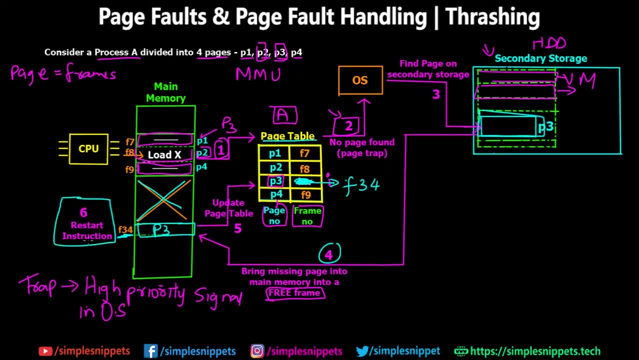 entire page. fault handling system is going to be sixth step, which is restart the instruction, which means that cpu is going to be again restarting load x and now it's going to find p3 in the memory, because it is found over here in the page table. so now cpu will start executing. 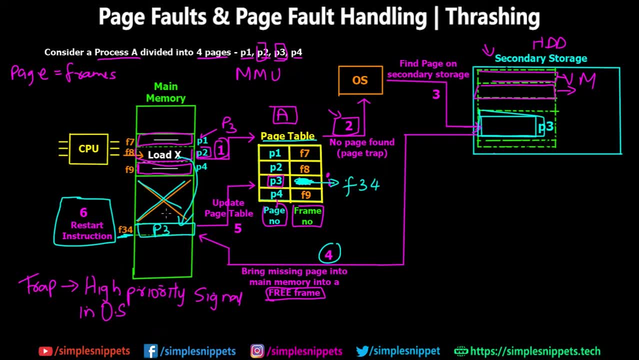 page number three. so this is the entire page fault handling scenario and all the steps which are there which i performed when a page fault happens. now note that if this p3 would already be located over here- so let's assume that p3 is already here and not here, that is, in f34 page fault would have. 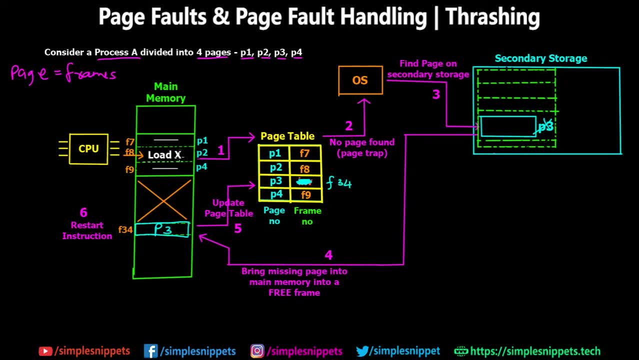 not occurred at all. right, cpu would have come to this instruction, load x, which would want p3. so the mmu would look up p3 in page table. it would come to this location, p3. it would say: okay, i have found the frame, that is frame 34, so directly from step. 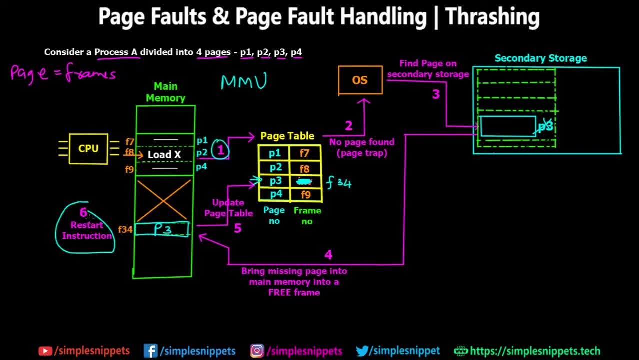 now step number six would be achieved because we've already found the frame in memory right. so p3 is already there in frame number f34, so it is already there in memory. so all these steps are not required. that is step number two, three, four, five, so directly the mmu will inform cpu that it. 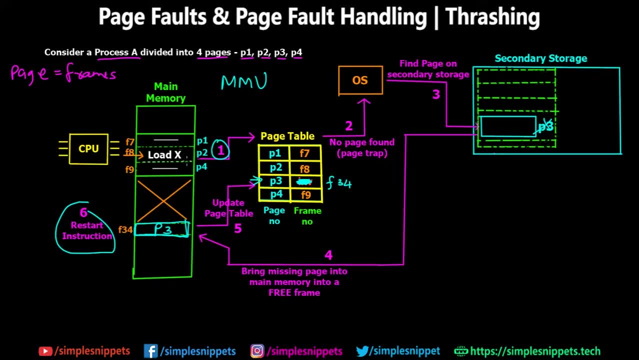 is there in the memory at frame 34 and cpu will directly come from frame 8 to frame 34 to perform or execute p3. okay, so this was page fault and page fault handling and by understanding this, let's try out a small numerical which usually comes in exams and 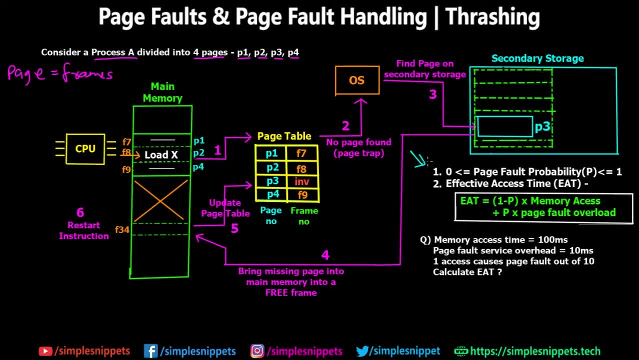 it is associated with page fault only. so this is some details regarding page fault. so point number one says zero less than equal to page fault probability, p less than equal to one. so when paging scheme is implemented sometime or somewhere, page fault is going to happen, right? so 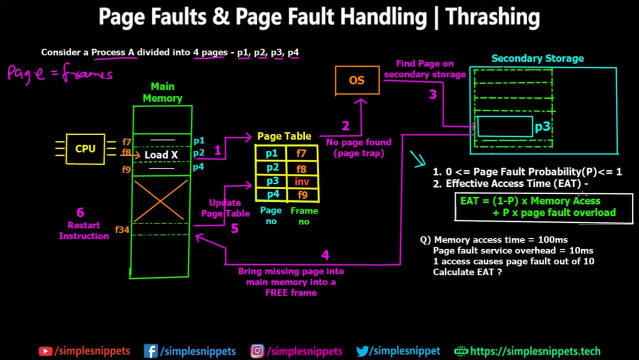 when the main memory is getting full, a lot of pages are being swapped between the main memory and secondary storage, so if certain page is not there in the main memory, a page fault is going to occur right, which means that the page fault probability is going to be between 0 and 1. 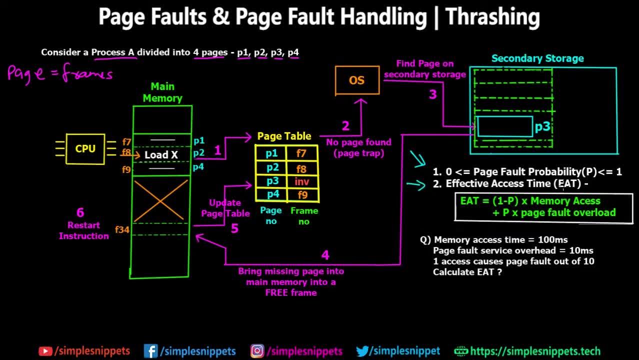 so point number 2 is the effective access time: e80. so e80, or effective access time, is the time required to access a particular memory address, to access a particular page, and the formula is given by e80 is equal to 1 minus p. so p is the probability of page fault happening. so 1 minus p is going to. 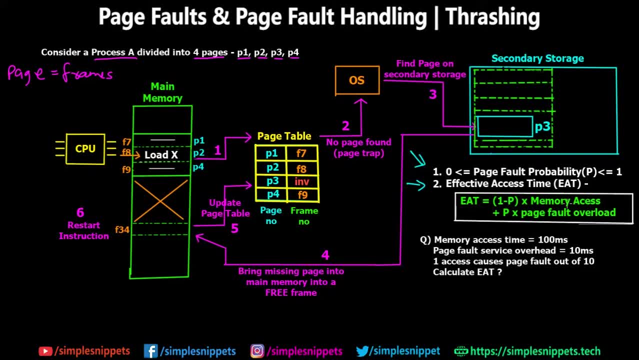 be the probability of page for not happening into memory access. that is, we got the page plus p into the probability of page fault happening, into page fault, overload or overhead. so whenever a page fault happens we have to go through step number two, three, four, five and six right and whenever. 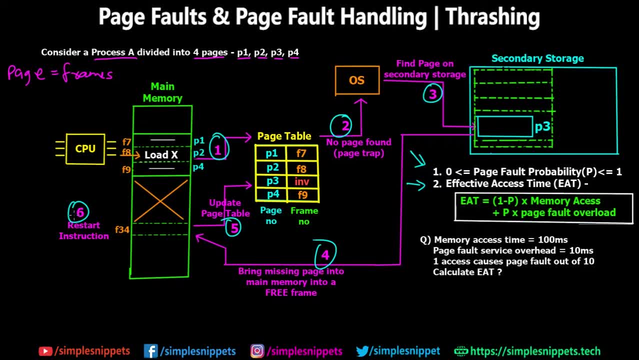 a page fault doesn't happen, we can directly jump from step number one to step number six. right? so this page fault overhead is the extra time required whenever a page fault happens to perform this step number two, step number three, step number four, step number five and step number six. okay, so this is. 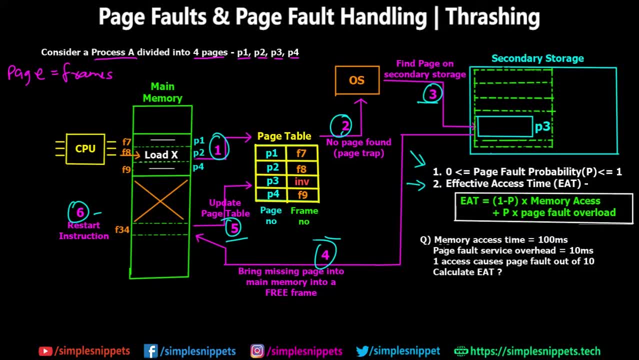 the probability of page fault happening into page fault overhead. so depending on all these details, we have a question. let's say the memory access time is 100 milliseconds. so in general the time required to access memory is 100 milliseconds. the page fault service overhead is 10 milliseconds. 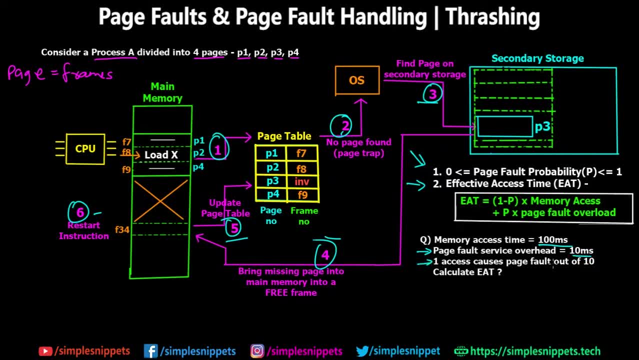 so whenever a page fault happens, 10 milliseconds are required extra. and the third detail is one access causes page fault out of 10, which means that the probability indirectly is given as 1 by 10. okay, one time a page fault happens so indirectly they've given us a probability only right. 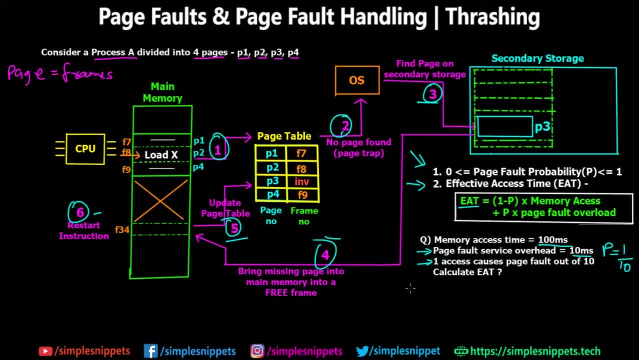 so using this formula of e80, we can say that e80 is equal to 1 minus p. so we know p is 1 by 10, which is 0.1. so this is 0.1. so 1 minus 0.1 into the memory access. so they already have given memory. 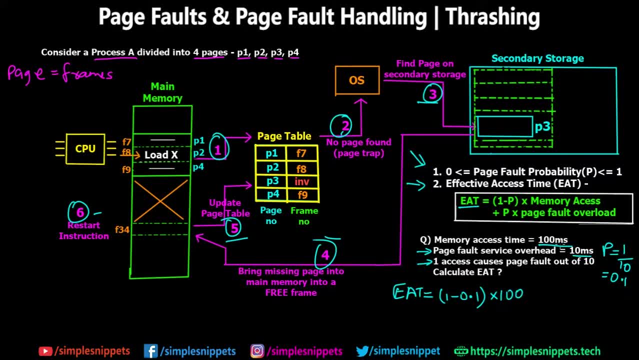 access time, which is 100, and this is in milliseconds. it can be in nanoseconds or microseconds, so make sure you do the conversions properly and get all these values in one single unit. so then we have plus probability, which is 0.1, into page fault overload, which is 10 milliseconds, so 0.1 into 10.. so solving this further: 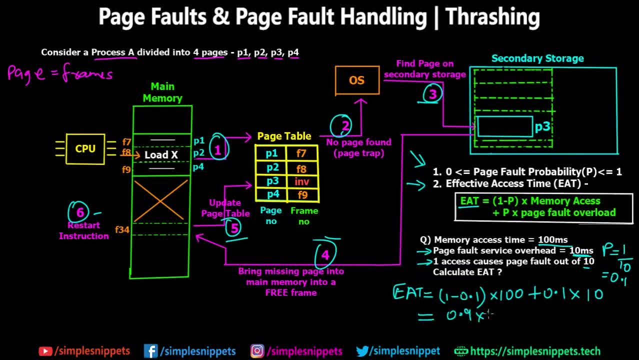 we have 1 minus 0.1, which is 0.9 into 100 plus 0.1 into 10.. so 0.1 into 10 is going to be 1 and 0.9 into 100 is going to be 90, so ultimately, 90 plus 1 is going to be 91 milliseconds. so this is the. 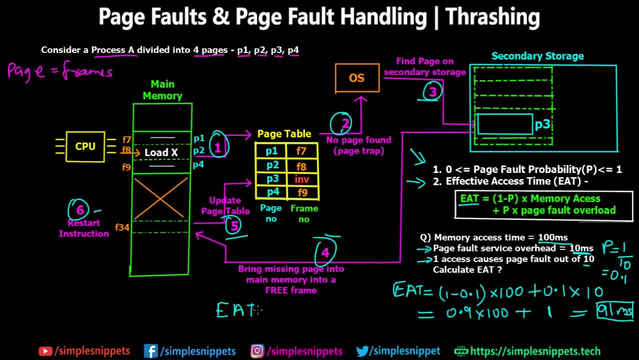 final answer 80 in this question is going to be 91 milliseconds. Okay, So I hope you have understood the entire concept of page fault and page fault handling, And we also saw a numerical as well as the entire working diagram of page fault handling. So, lastly, I just wanted to talk about the concept of 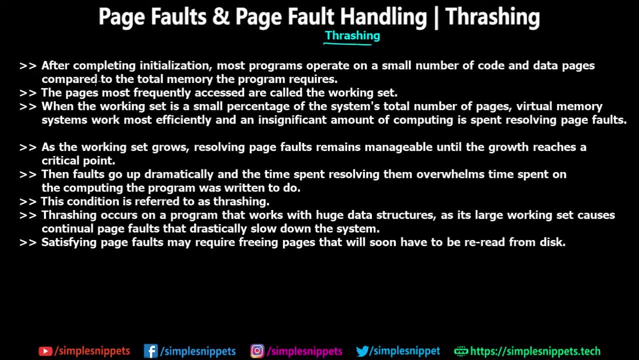 thrashing. So what exactly is thrashing? So let me just read out this theory and you'll easily understand. So, after completing initialization, most programs operate on a small number of code and data pages compared to the total memory the program requires. So what this point is saying is: 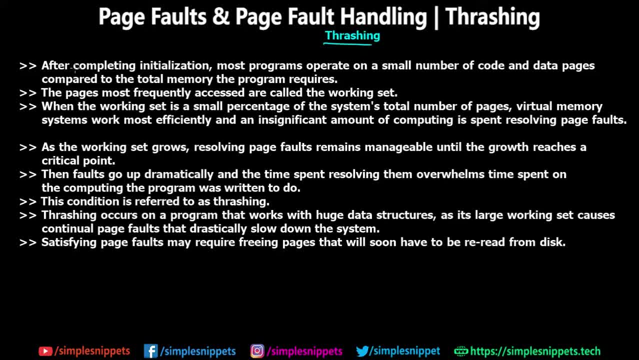 whenever you first time load a program, it takes a lot of time right. So when you initiate or when you start a program, there are a lot of things that are started and there are a lot of processes and background tasks required to initiate a program. However, once you start the program, 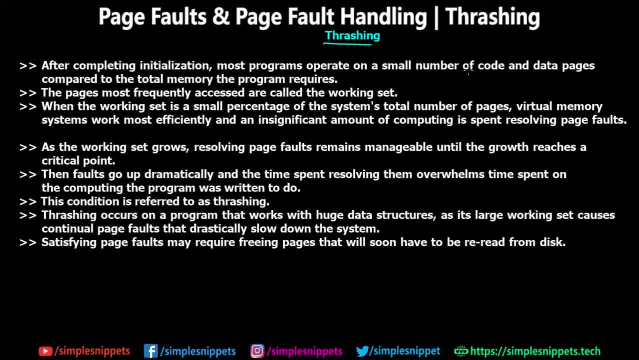 only a small number of code or only a small number of processes are running in the background, right. So take an example of a very high intensive graphic game. So when you start that game, initiate a program- it takes a lot of time. So when you start a program, it takes a lot of. 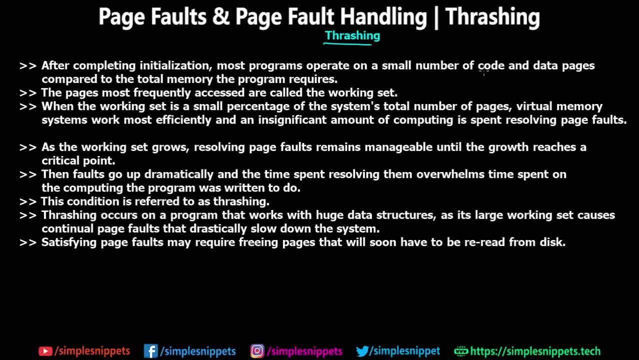 time right. But once the game is loaded, everything runs smoothly. So this you can make some analogy to this point. Now the pages most frequently accessed are called working set, So the most frequently run processes in the background for a particular application and 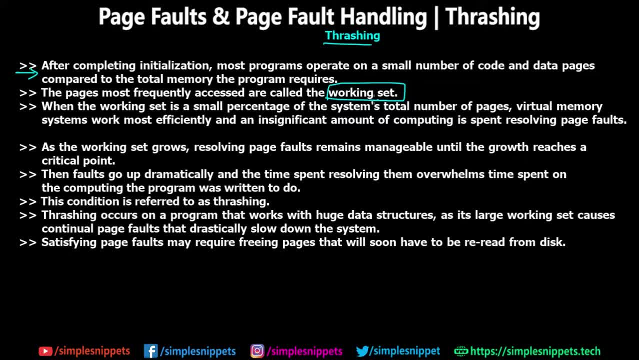 the pages that are most frequently accessed for those processes are called as working set. So in the working set is small percentage of the system's total number of pages. Virtual memory system works most efficiently and an insufficient number of pages is a small percentage of the system's total number of pages. 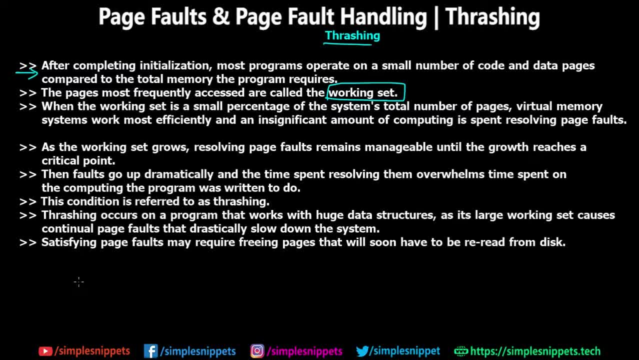 So if you're on a computer, you will see that a very small percentage of the system's total number of pages is spent in a way that is considered much more beneficial than a physical application, Because if you're on a computer, you will see that a rather insignificant amount of computing is spent. 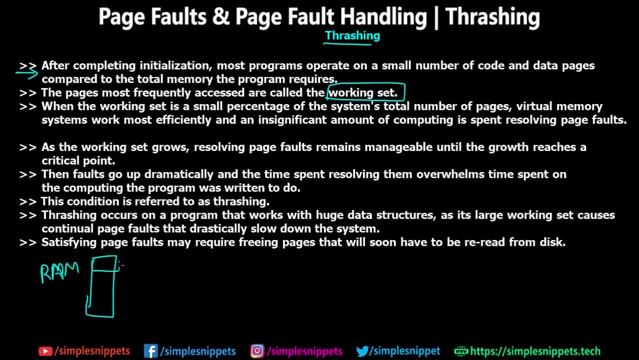 and you will also see that a rather insignificant amount of computing is spent resolving page faults. So what they're saying is: if you are Ram, this, so this is. Ram has a very small amount of this working set of pages, so there won't occur a lot of page faults, right? So this is the virtual memory VM and this is the physical memory Ram. 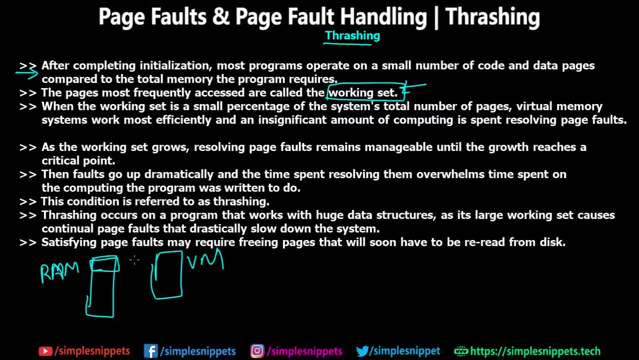 So when this working set is small they won't occur a lot of page faults because there won't be pages being swapped between virtual memory and RAM. But as the working set grows, so as the RAM gets filled in gets filled up with all these working set pages. some pages are being transferred to the virtual 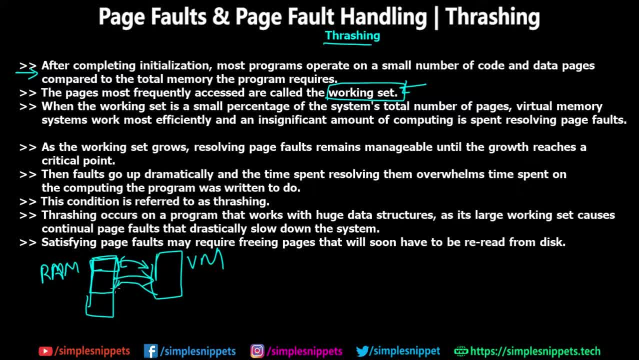 memory and then, when they are required back again, they are brought back into the ram. so as the working set grows, resolving page faults remains manageable until the growth reaches a critical point. so this page faults happen again and again as the working set grows. okay, so as the ram fills.